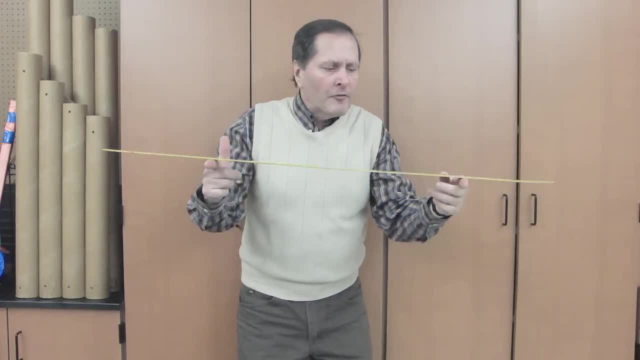 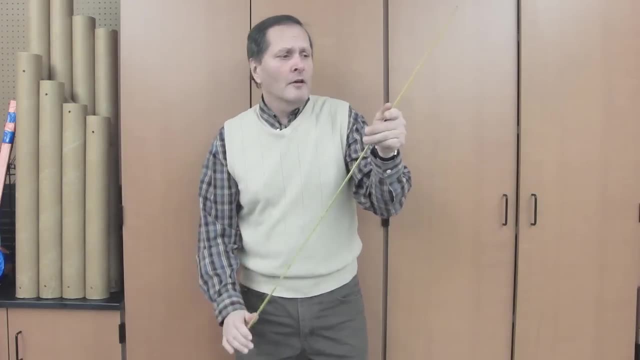 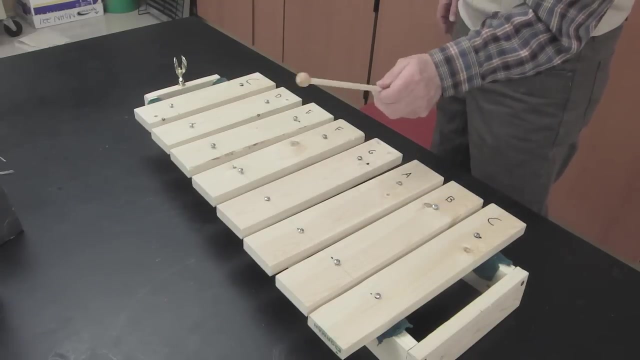 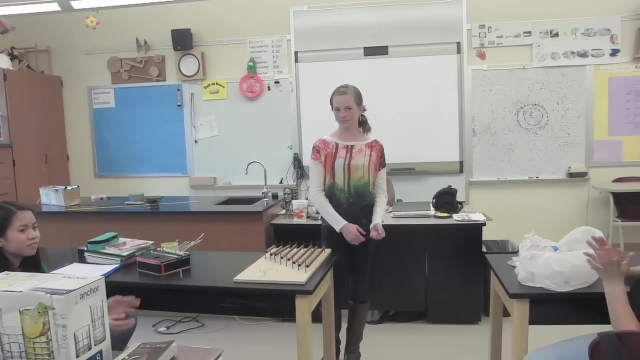 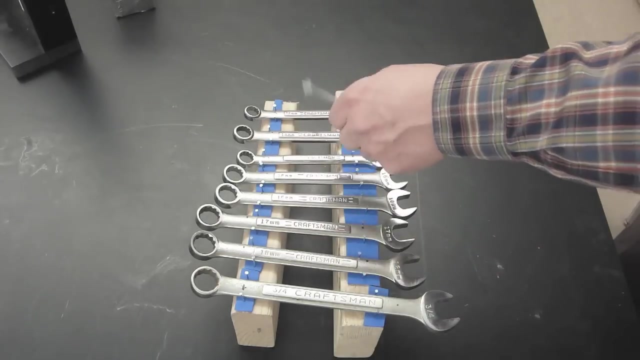 And if the bars are supported at about these positions, it's going to give us a much better sound than if you tried supporting it somewhere else. 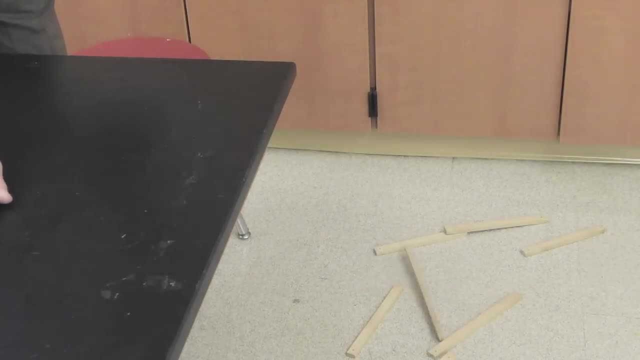 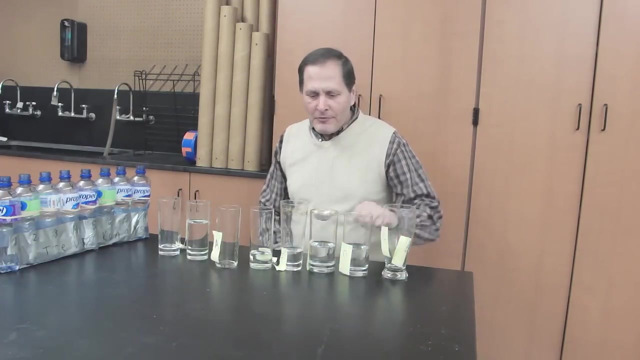 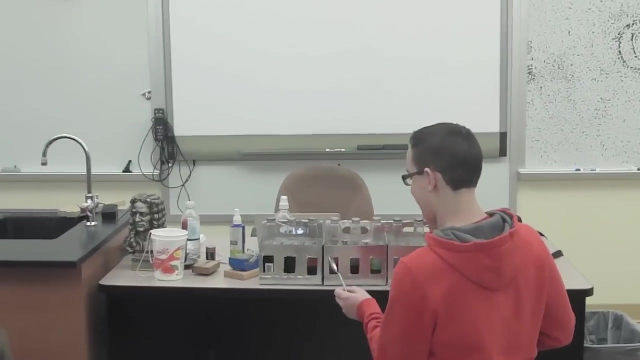 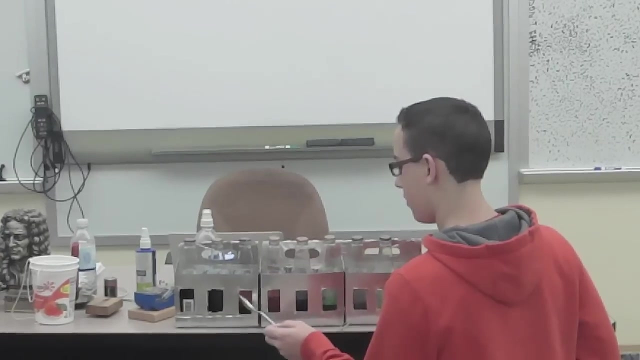 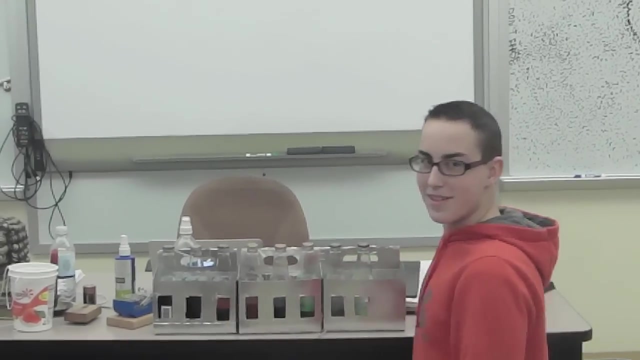 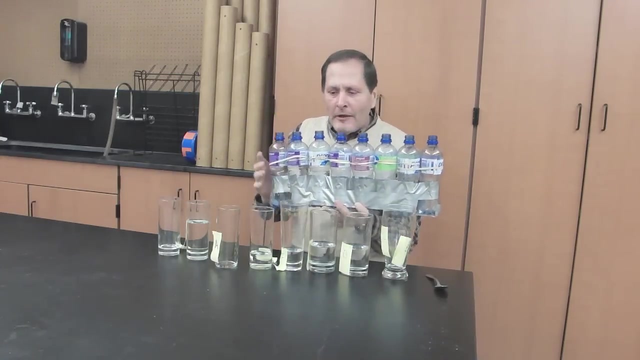 Now another popular idea is to use various size containers filled with water and we strike them with a hard surface to get different sounds. Or in this case, we have same size bottles filled with different amounts of water and we blow across the opening at the top. 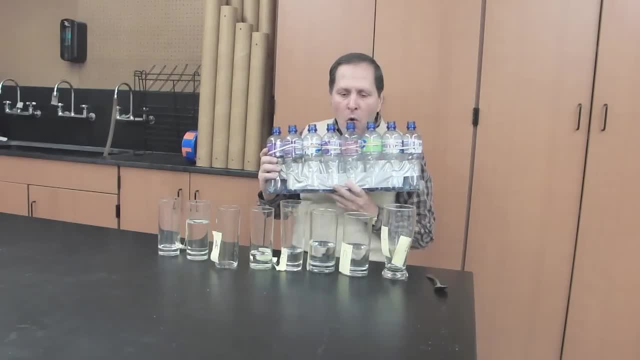 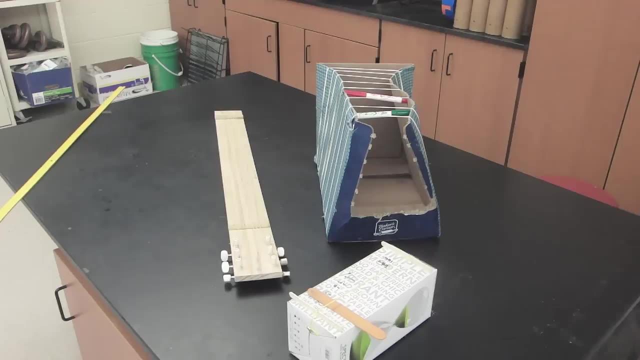 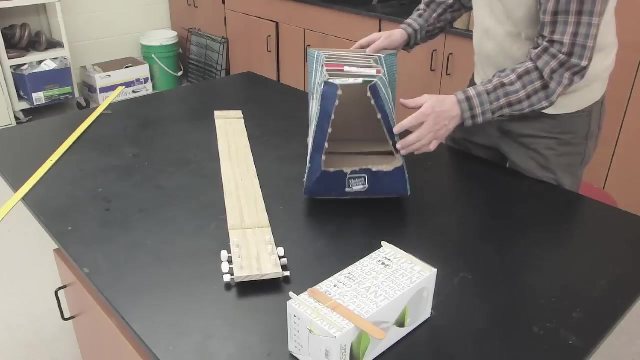 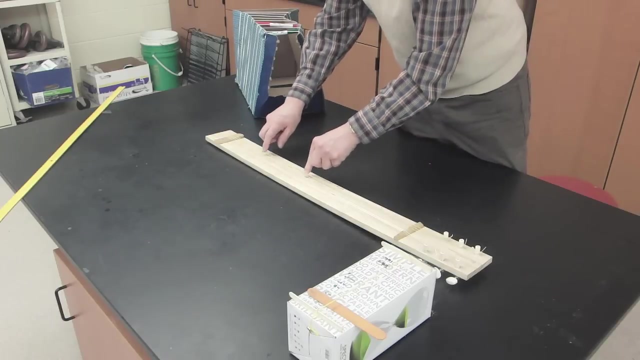 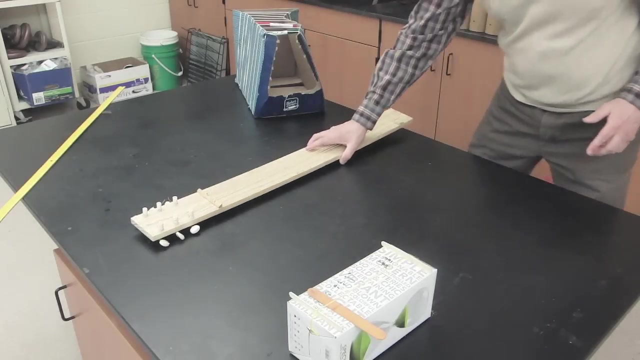 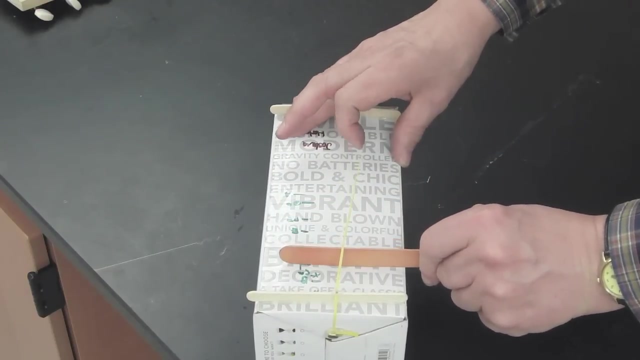 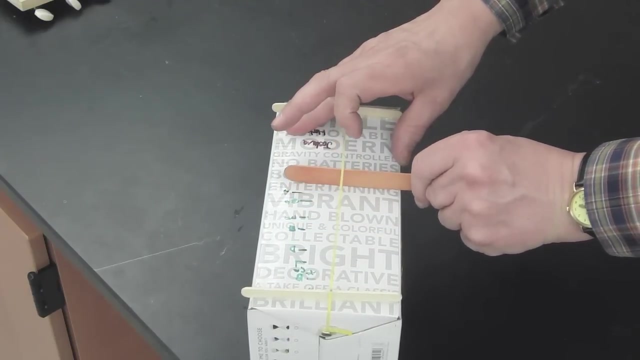 Yeah, that's always fun. Now we had a variety of stringed instruments. in this case it was rubber bands. This piece was similar to a guitar setup, And in this next piece, the pitch was changed by changing the position of the bridge. 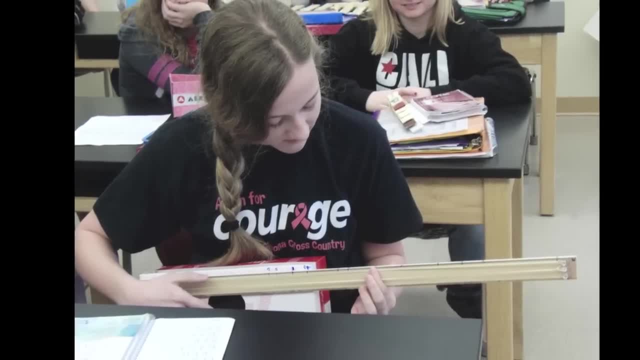 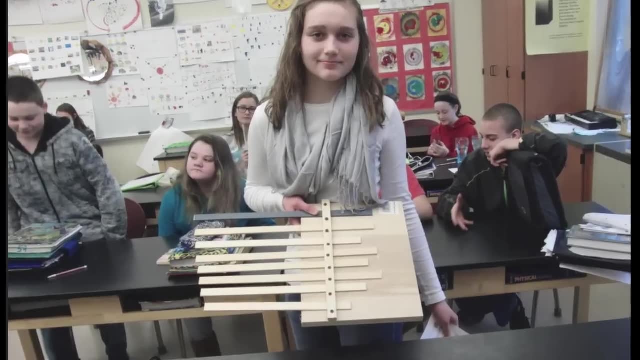 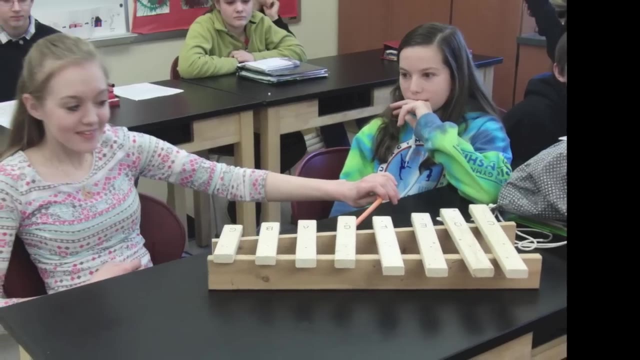 So here are a few more of the ideas that my students came up with. So here I have done a mixture of blue, white and brown. Now these are some of the touches that I have used With the blue, white and green. this is what I have done. 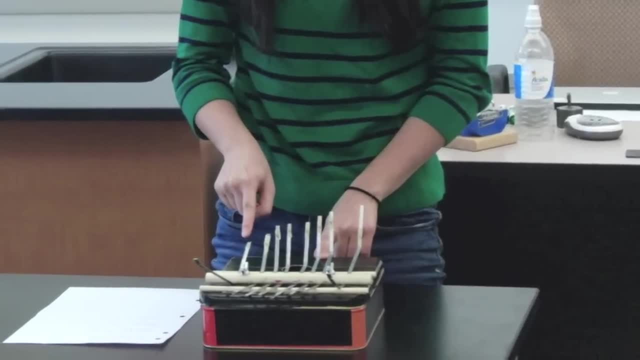 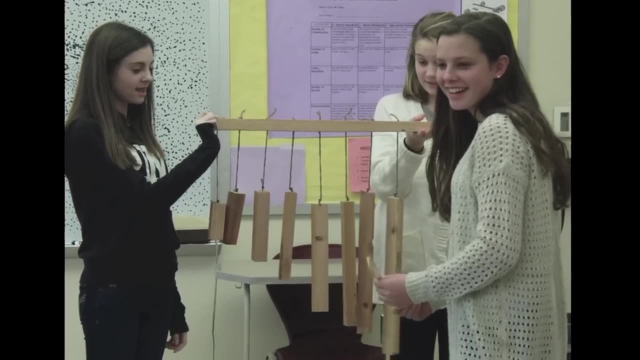 It can be used to create a kind of string that has a little bit of a sound, And I have added blue, white and blue. Now what I can do is I can add the color and I can also add the sound effects. So here I have done a few notes. 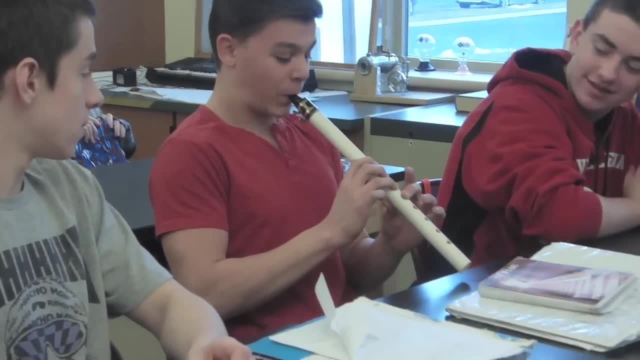 So this is how I have chosen the colors, And I just then added the consistency, I added different tones and then I added the credits, I added the white in the middle of the strings, in the middle of the strings, And I just added a little bit of the red and blue.